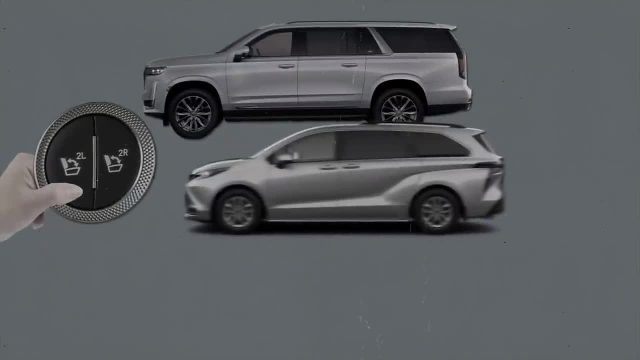 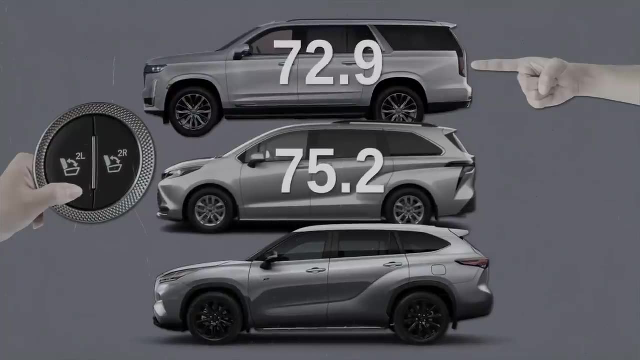 just 16 cubic feet. but let's say you fall down the third row seats in all three vehicles. the sienna escalade gives you 72.9 cubic feet, whereas the highlander gives you 48.4 cubic feet. so here again. the minivan wins. but now let's fold the second row seats. i'm talking an impressive 101 cubic feet of cargo space in the sienna, but here's where the escalade gives you more, at 121 cubic feet again. the loser here is the highlander, which only offers 84.3 cubic feet, which is nowhere near. 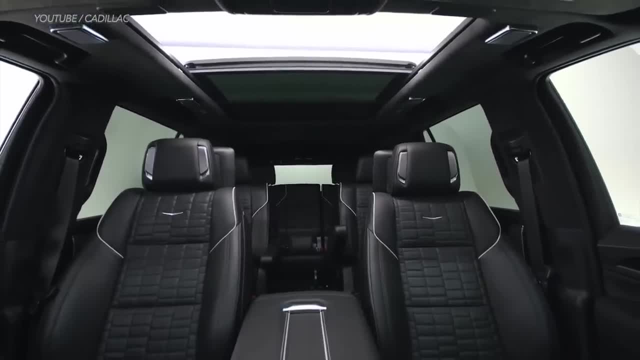 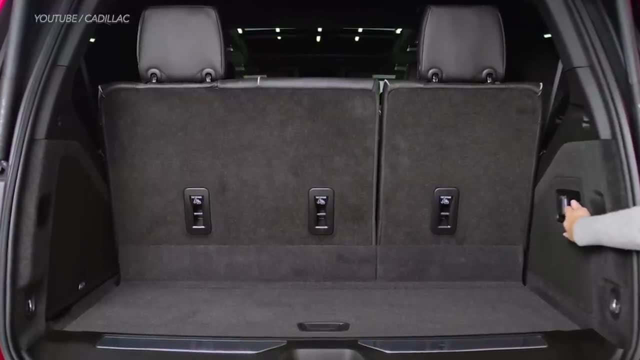 the other two cars. side note: if you look at the long wheelbase cadillac escalade esv you'll find cargo space across all combinations. i'm talking 41 and a half cubic feet of room behind the third row, or 94.1 cubic feet with the third row folded down, or 142.8 cubic feet with the second row. 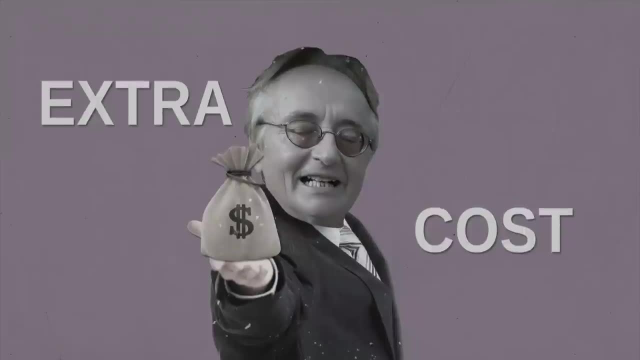 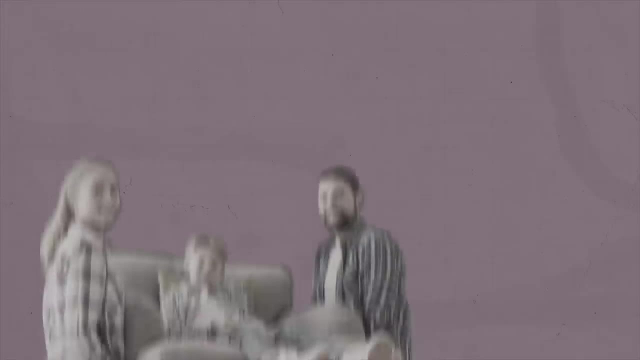 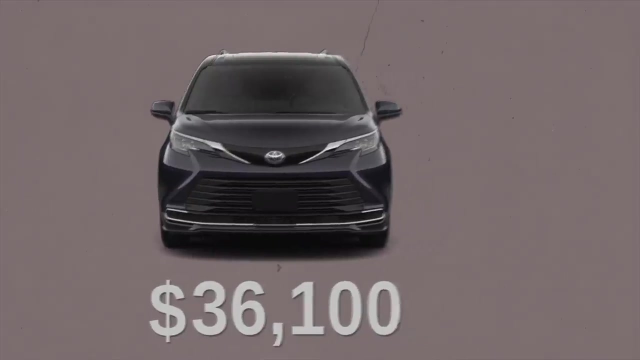 folded down, but that all comes at an extra price tag. the high performance escalade v starts at a whopping 149,195 bucks, so if cargo space is your priority, consider this. the sienna starting msrp is just over thirty six thousand one hundred, where the escalade v starts at. around 149,200,. in other words, is that extra cargo space and a long wheelbase escalade v worth an additional hundred and thirteen thousand one hundred dollars? for the most part, i'd say the answer is no bottom line. the minivan's cargo space should meet the average american's need. 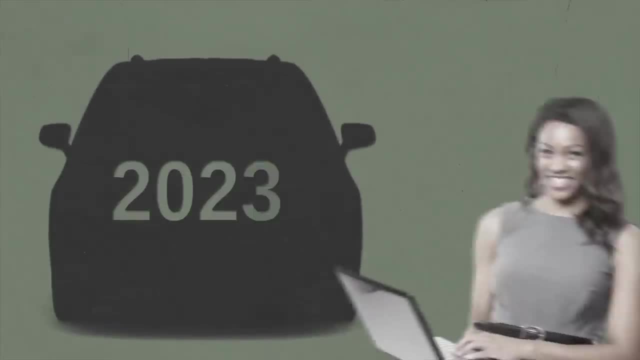 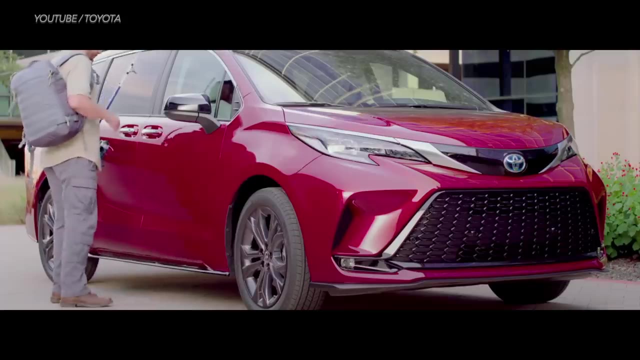 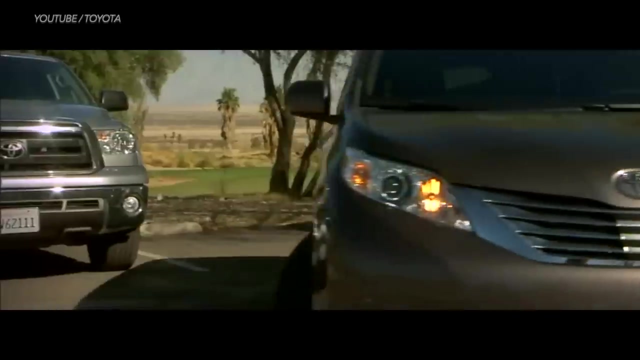 while keeping things in budget. in fact, believe it or not, every 2023 minivan on the market right now has more cargo room than a ford f-150 truck bed. don't forget sliding doors. you might think it just slides open automatically and effortless. your kids can't scratch or bump the car next to. 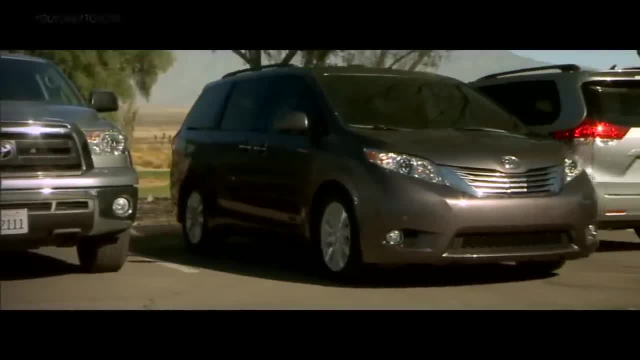 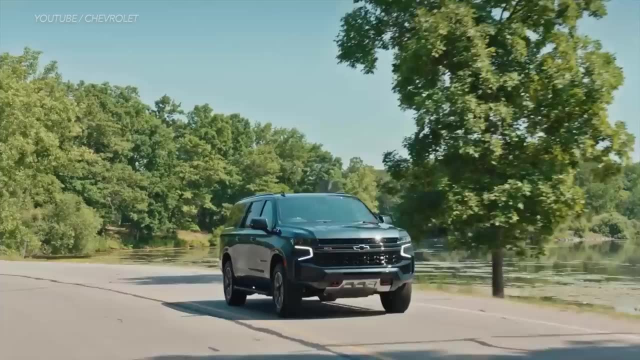 you. this is one of the hallmark features of a minivan that you can't find in popular crossovers or suvs. but now let's talk about gas mileage. an suv, especially a full-size one- it's huge and it eats up a lot of gas. the trade-off of having a bigger engine that outputs more power is that. 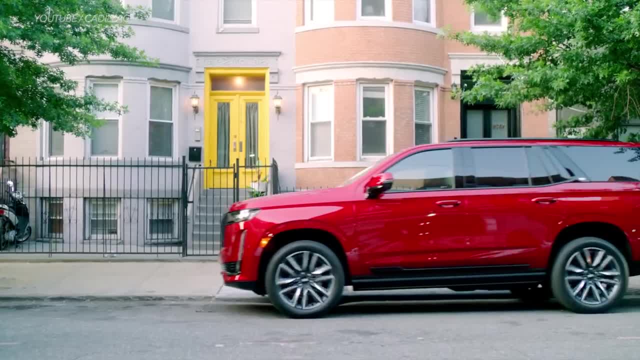 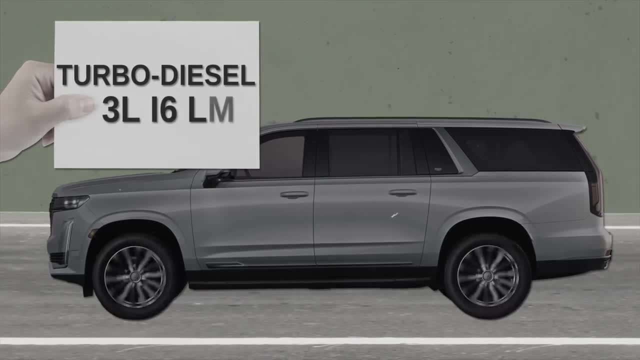 it requires more fuel to be burned. don't even get me started on the gas mileage of the cadillac escalade. a 2023 cadillac escalade with a turbo diesel, three liter i6 engine, lm2 powertrain has a gas mileage of just 20 miles a gallon in the city and 26 on the highway. 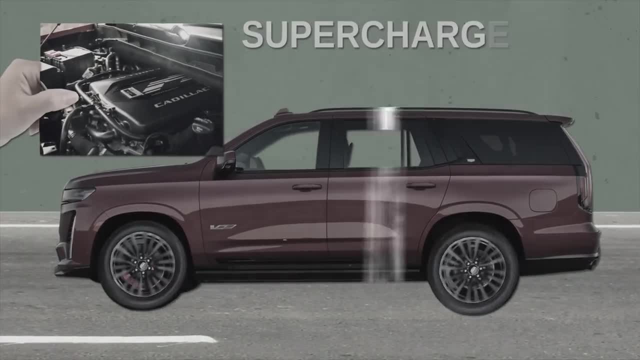 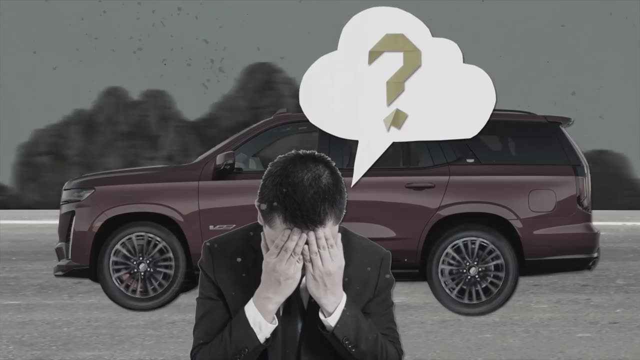 but here's even more shocking: the escalade v with a supercharged 6.2 liter v8 lt4 powertrain will get you a mere 11 miles a gallon in the city and 16 miles on the highway. now a minivan on the. 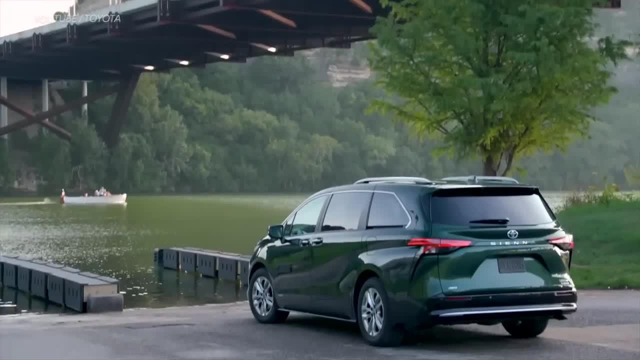 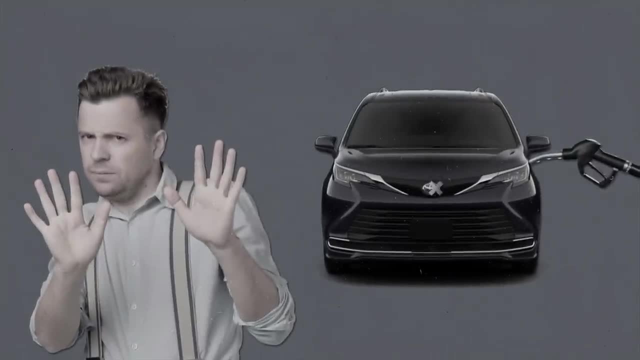 other hand, is lower to the ground and drives more like a car. because of its engine, the minivan usually has better gas mileage compared to an suv and crossover competitors. toyota stopped offering gas-powered siennas starting with the 2021 model onward, so 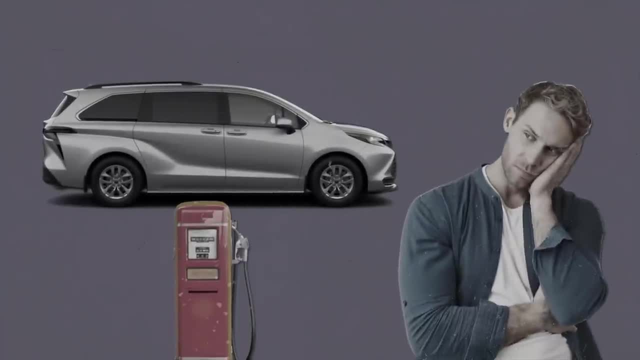 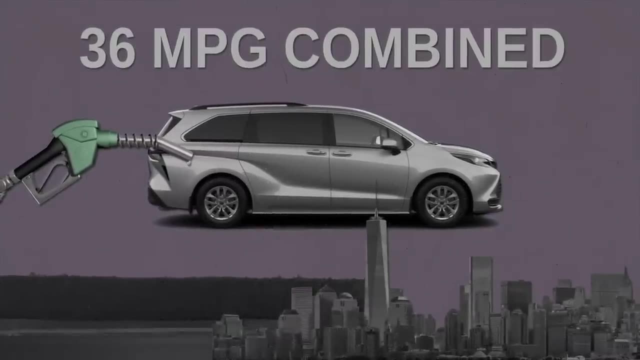 for the 2023 sienna minivan, you'll see it comes exclusively in a hybrid powertrain. the front wheel drive version has an epa estimated gas mileage of 36 miles a gallon, both in the city and on the highway. if you want to compare that to a gas-powered toyota highlander, well, the gas 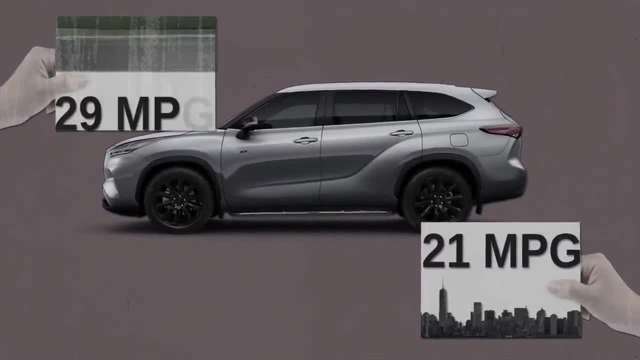 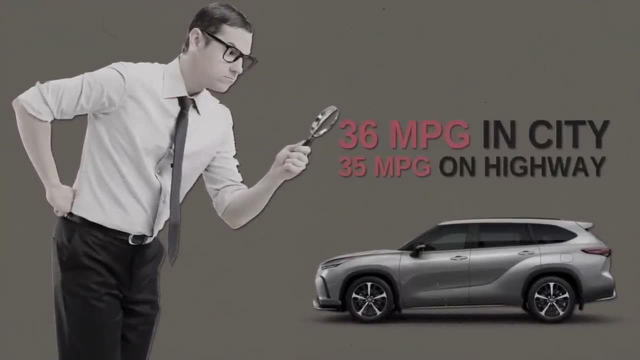 powered, one gets just 21 miles a gallon in the city and 29 on a highway, so that puts it out of the race. the hybrid four-wheel drive version offers 36 in the city and 35 on the highway, so it's fairly comparable to the minivan. the average minivan costs less than a 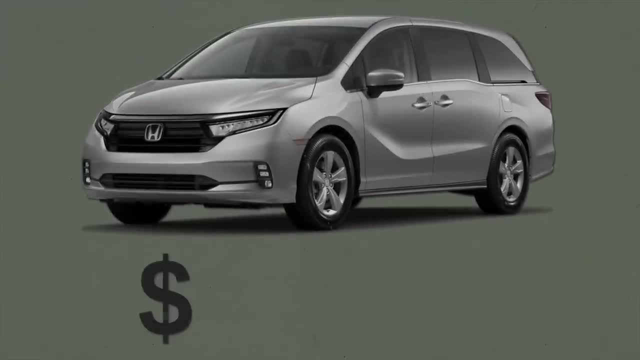 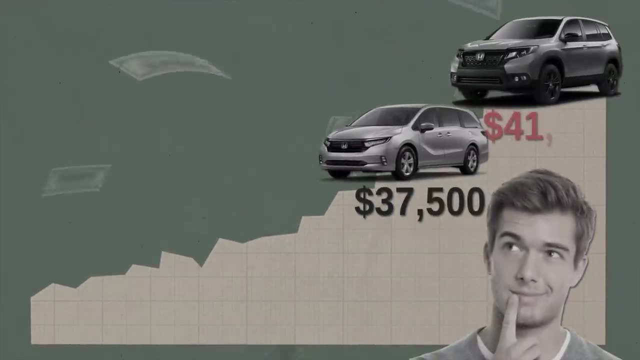 three-row crossover. honda odyssey minivan, for example, starts at 37 500, which is three thousand six hundred dollars cheaper than the honda passport midsize crossover, starting at forty one thousand one hundred dollars. on the other hand, the toyota sienna starts at thirty six, one, three, five, which 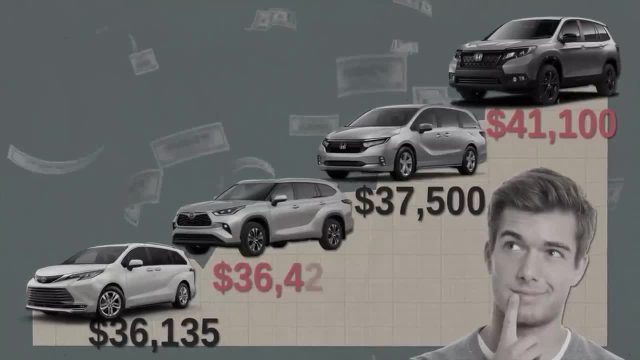 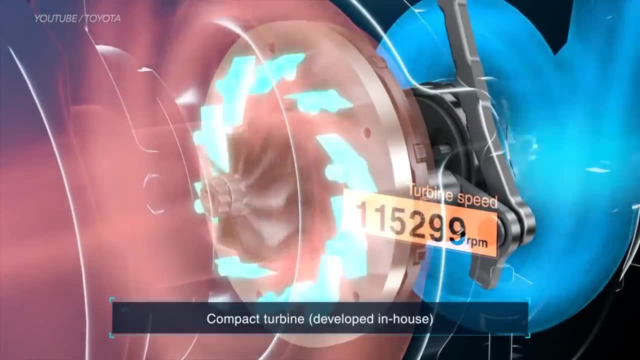 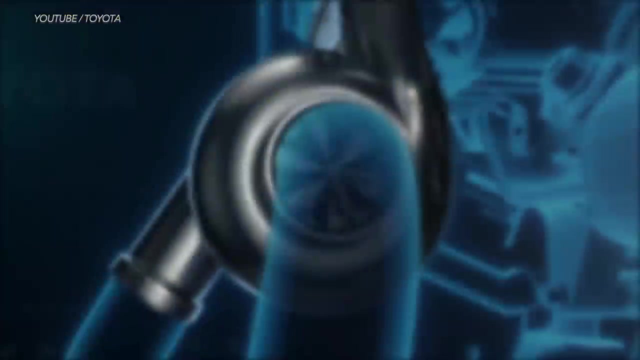 is just 300 bucks cheaper than the highlander, which starts at thirty six thousand four hundred and twenty dollars. now let's talk about turbocharging. a turbocharger gives an engine extra power without sacrificing fuel efficiency. usually turbochargers are the smaller engines to improve performance. basically, a turbo compresses exhaust gas and 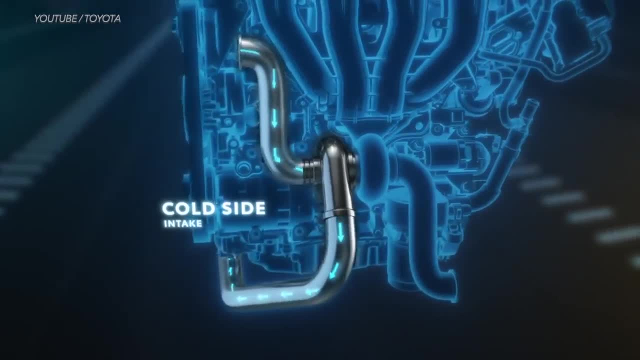 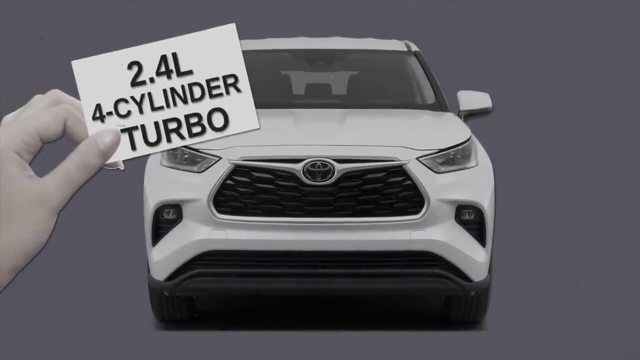 then sends compressed air back into the engine. this increased airflow sends more fuel to the engine, which outputs more power. the highlander xle trim comes with a 2.4 liter four-cylinder turbo engine. the thing is typically: a vehicle with a turbocharged engine is usually a bit more. expensive than one with a naturally aspirated engine. also, many turbocharged engines require premium gas. a turbocharged engine isn't always as reliable as a naturally aspirated engine. just more parts of an engine, the more can go wrong. turbocharged engine usually requires more routine. 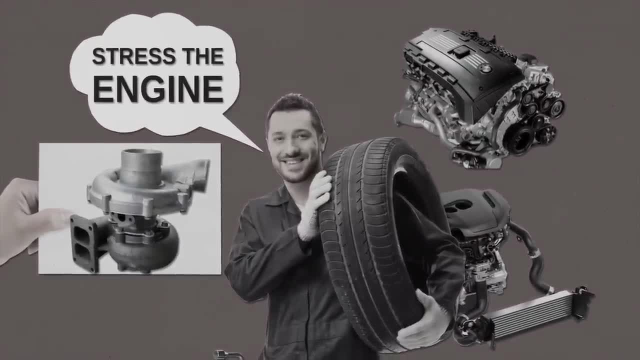 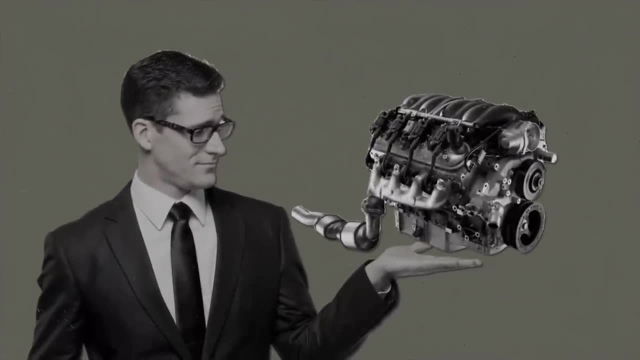 maintenance, because turbochargers stress the engine and its parts. if you're planning on hauling heavy loads, a turbo boosted smaller engine is not the best way to go in most cases. it's just better to get a bigger engine. now, the toyota sienna does not come with the turbo option but, honestly speaking, 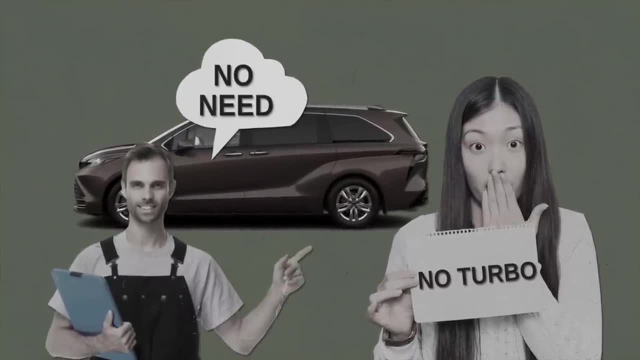 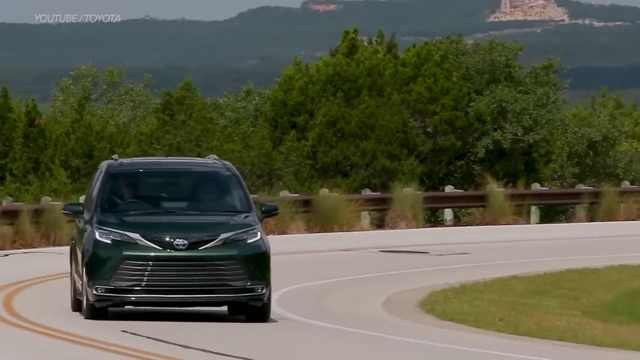 when it comes to a minivan. while it is possible to turbocharge your minivan, there's really no need to, and that saves you a world of trouble in the long run. minivans will also save you money on car insurance. there are a few reasons why it's generally cheaper to insure a minivan as opposed. 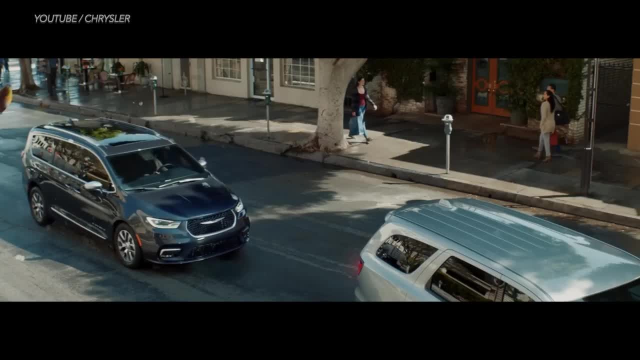 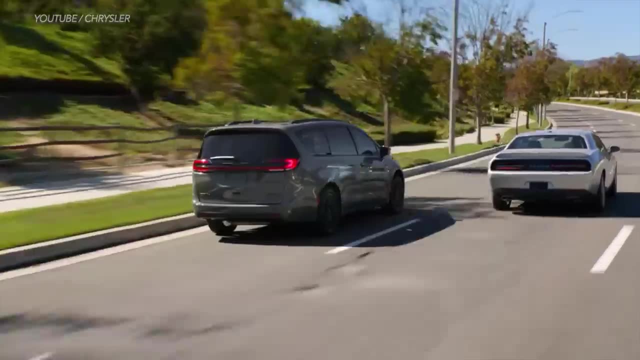 to an suv. first of all, statistically speaking, minivans aren't in as many accidents. the average minivan driver is usually a lot more cautious on the road compared to other drivers. part of it comes down to the fact that there are children in the back, but it's also because the average minivan 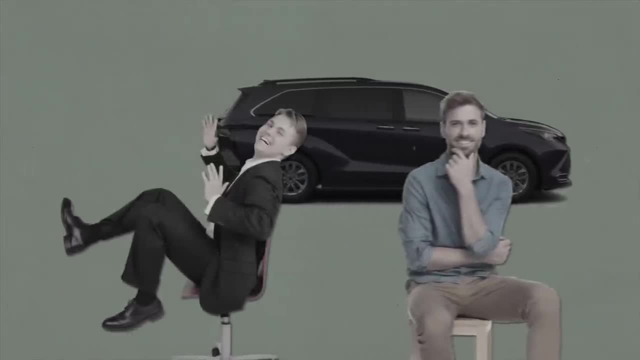 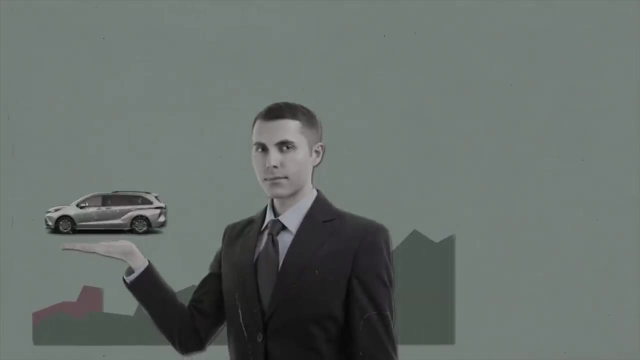 driver is demographically older and are more experienced drivers than owners of suvs, who are usually younger and less experienced as a group. another reason why car insurance costs are low for minivans is vehicle theft, and vandalism is uncommon with minivans. here you have the advantage of the. 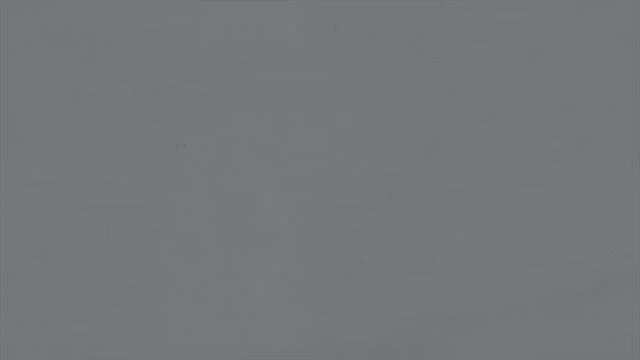 minivans being less popular than crossovers and suvs. less popular means you're not on the top of the list among vehicle thieves, and that translates into low insurance claim risk. minivans also have higher safety ratings, and that translates to lower insurance premiums. last but not least, 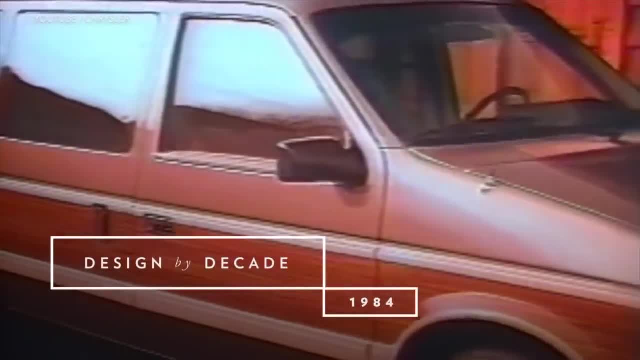 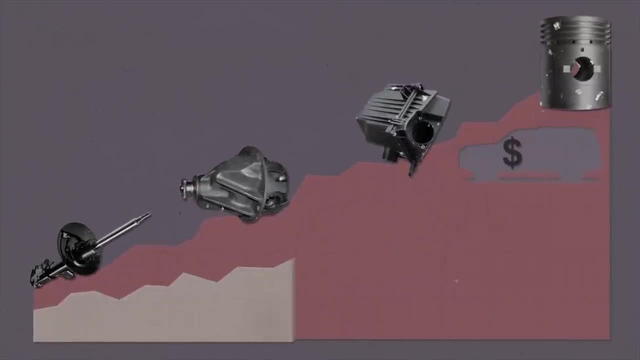 minivans have been around for decades and are rather common, so if you need to repair or replace a part, the parts are typically accessible and easy to source. so parts replacement costs are lower compared to crossovers or suvs. car insurance companies like that if a car part is easily. 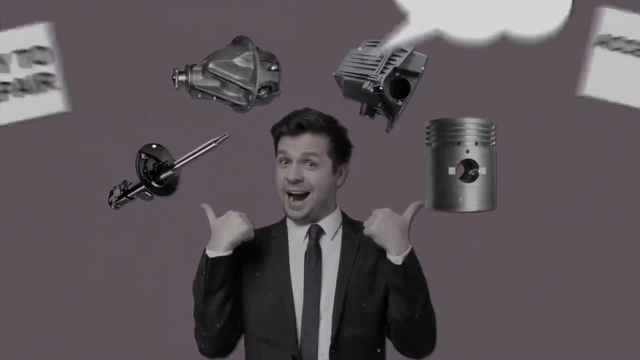 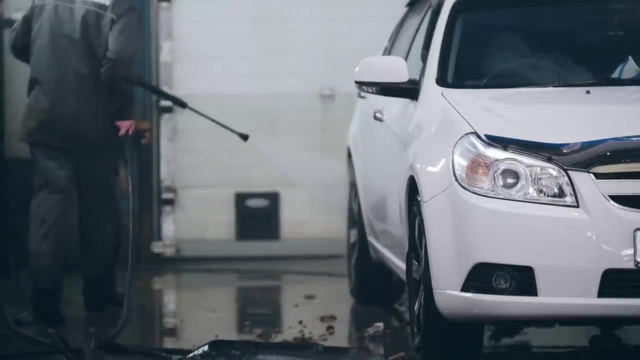 accessible and less expensive to repair. that vehicle has a lower cost risk to the company and that's why you enjoy lower insurance premiums. here's another advantage to minivans: car washing costs. many car washes charge more for larger vehicles. in many cases it's cheaper to get your. 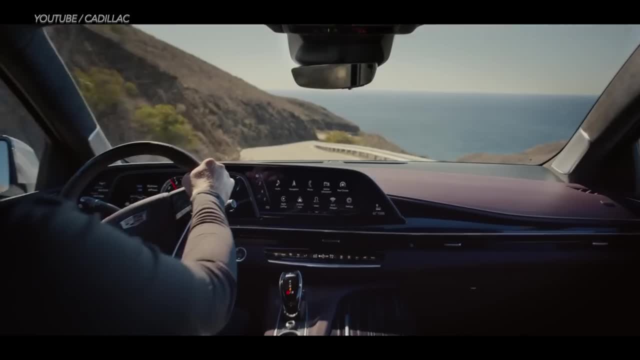 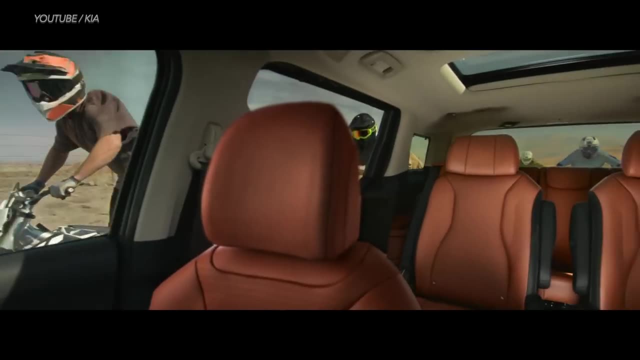 minivan wash compared to a full-sized suv, but let's shift gears and talk about safety. when it comes to driving, visibility is an important fact. obviously, the more you can see ahead on the side and the rear the better, especially when you're changing lanes, merging into a highway or even 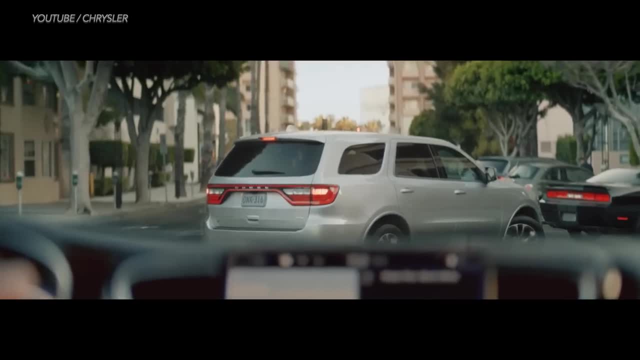 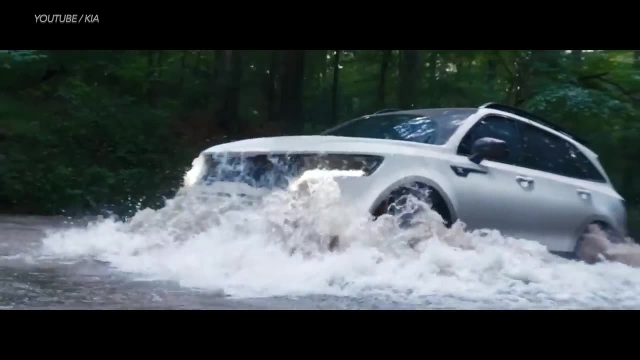 maneuvering into a parking spot, the minivan offers better visibility for the driver compared to the suvs. part of the reason is the lower ride height of the minivan, whereas suvs are taller, ride higher and have more ground clearance, higher hoods and higher bumpers. did you know that back in 2009,, one 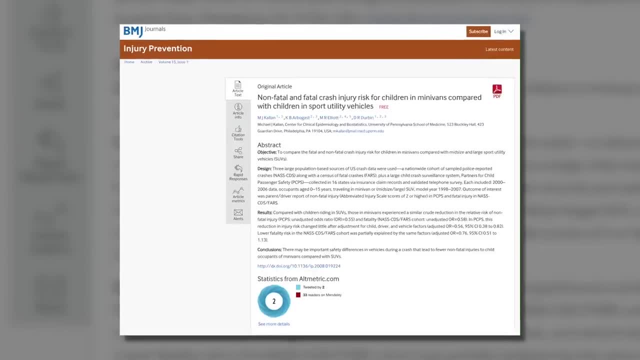 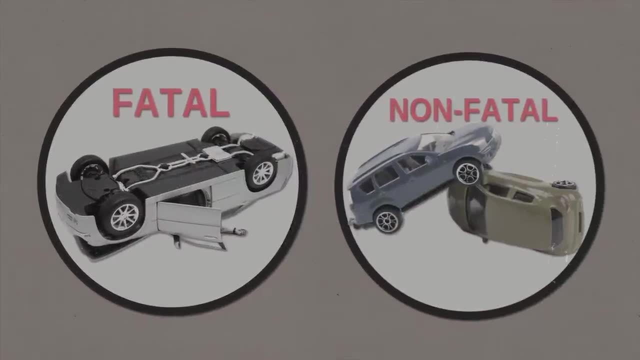 study found that children were less likely to be killed or injured in a crash if they were riding in the minivan as opposed to an suv. researchers looked at fatal and injury-causing crashes between 2000 and 2006,, and they found that children in minivans are 35 percent less likely to be hurt. 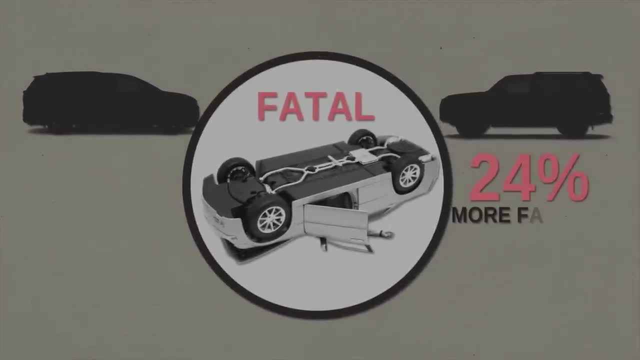 than children in an suv and in fatal crashes, there was a 24 percent greater chance of a child being killed in an suv than in a minivan. in that same study, a whopping 66 percent of suv fatalities involved a rollover, while only 37 percent of the minivan fatalities involved a rollover. 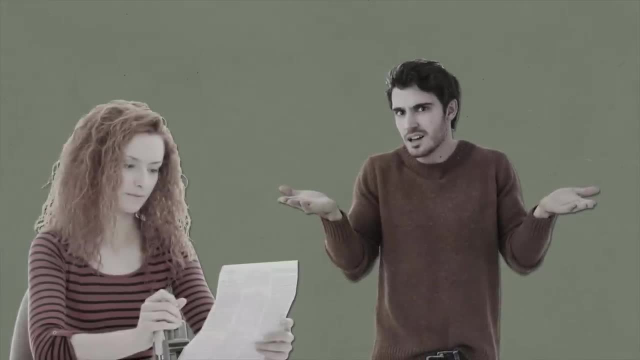 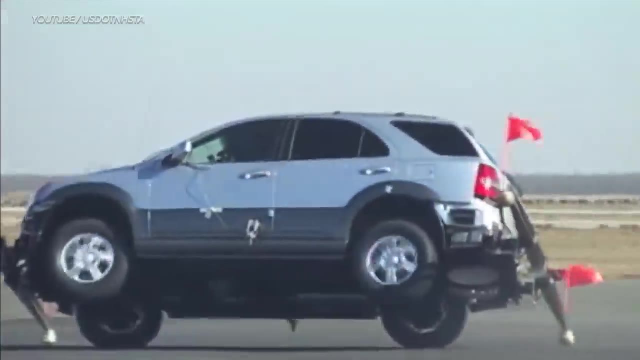 now. it's true that the study was done a while ago and suvs have improved since then. nevertheless, even today, minivans still have a lower rollover risk compared to suvs, so that's another safety factor you may want to keep in mind. 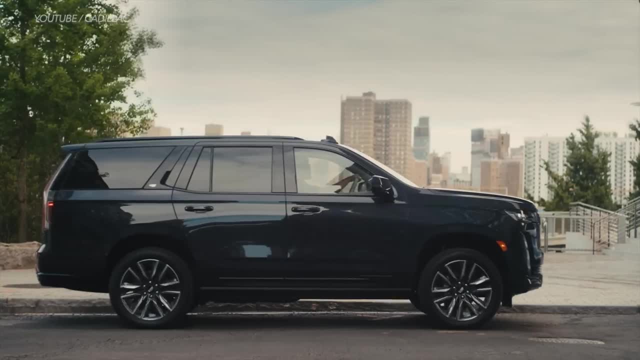 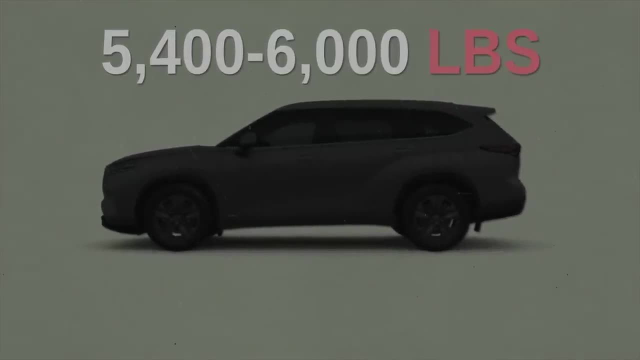 that said, when it comes to suvs, its large size and heavy weight is both a safety advantage and disadvantage, a blessing and a curse. the average suv weighs between 5,400 to 6,000 pounds. in some ways, suvs can provide better protection to its passenger inside than to a minivan, which 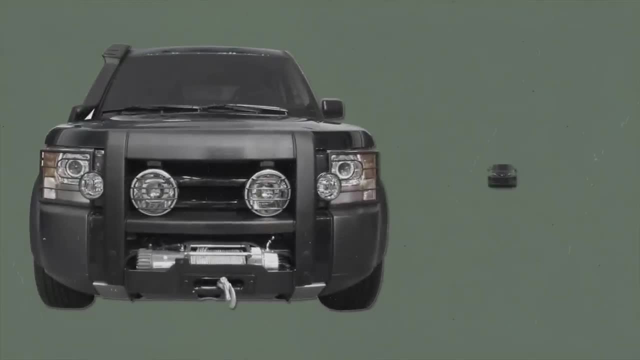 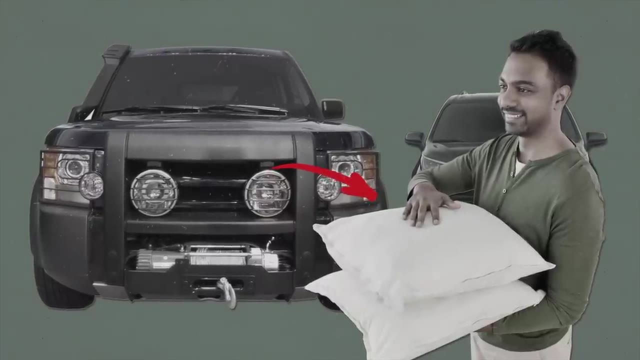 weighs less. for example, suvs generally have more reinforcement than a minivan and the heavy front bumpers function as crumple zones to absorb the energy from an impact, almost acting like a cushion, so to speak. on the flip side, its large size, heavy weight. 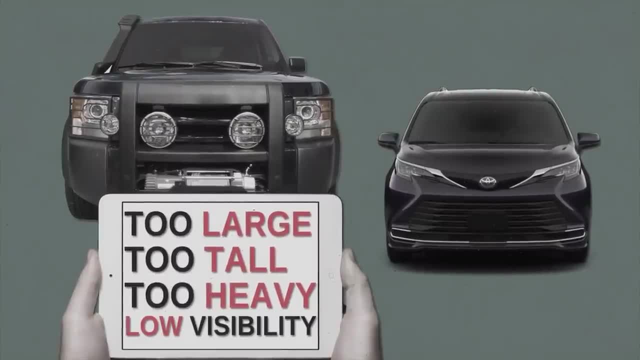 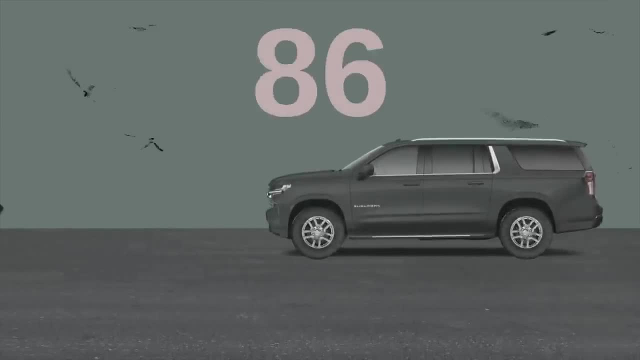 tall height, relatively low visibility are collectively also what causes more fatality to pedestrians and drivers and other cars when suvs are involved in a collision. by the way, I have a separate video that talks more about how suvs are killing us here in America, so check it. 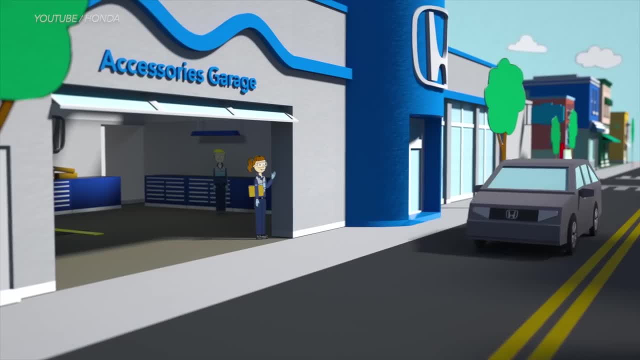 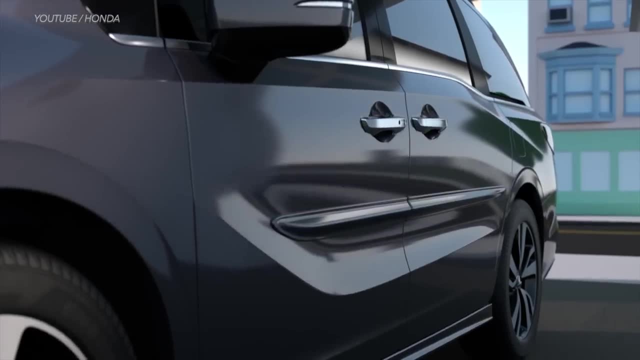 out anyway. in conclusion, minivans win categorically in most of the practical aspects that I addressed today. they just offer way more than crossovers and suvs. in certain respects, well, everything except the coolness factor. but how important is the coolness factor? 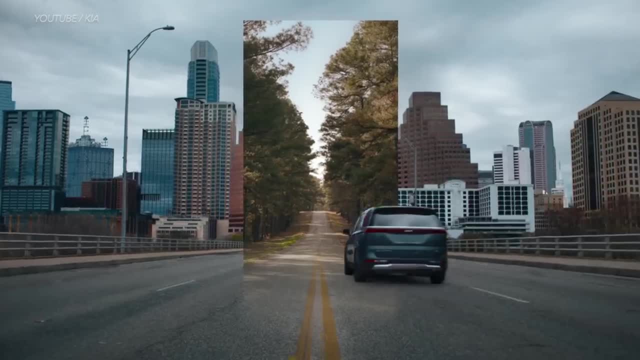 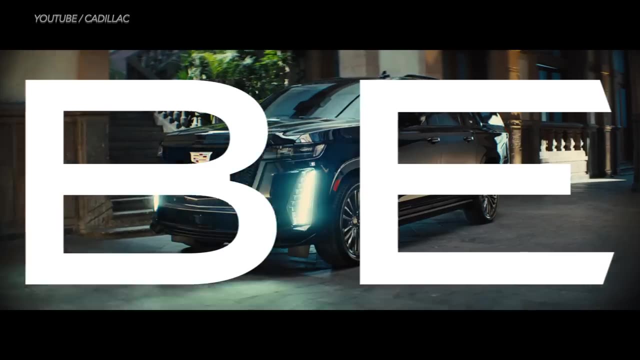 anyway. all in all, we should learn to be content with minivans. it's tried and true and steady. the thing is: in the past mothers helped make minivans popular in its day, but most moms care about looks and they like to follow fashion. mothers today don't want to be associated with